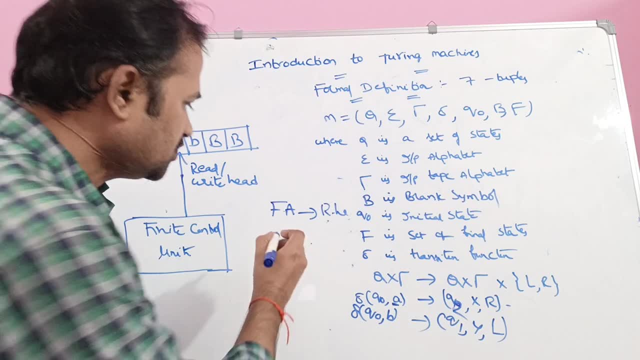 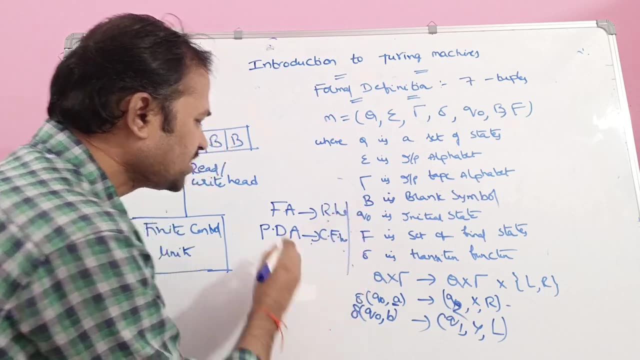 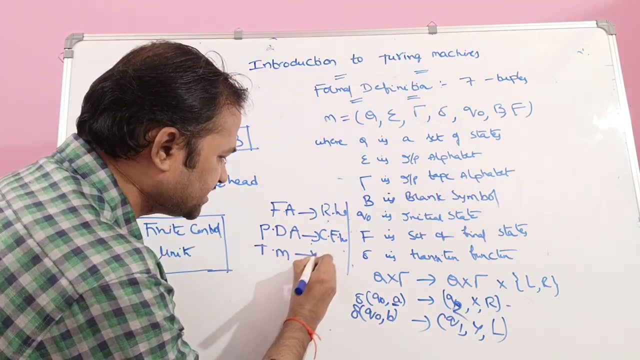 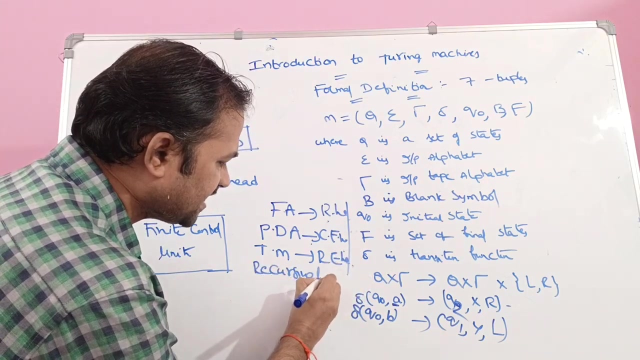 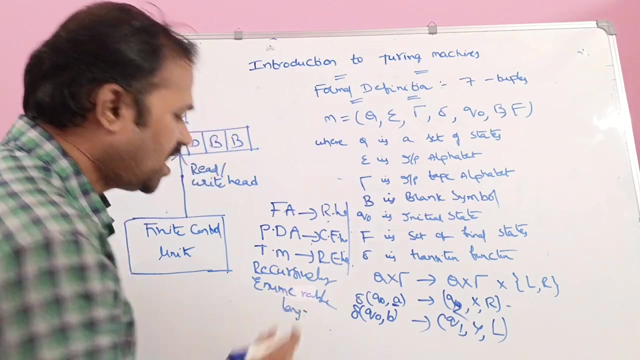 automata is called as context free language. So pushdown. automata accepts and recognizes context free languages. So likewise, Turing machine accepts and recognizes recursively enumerable languages. Turing machine accepts and recognizes recursively enumerable languages. Ok, First let us see here what is the need of. first let us see what is the need of Turing. 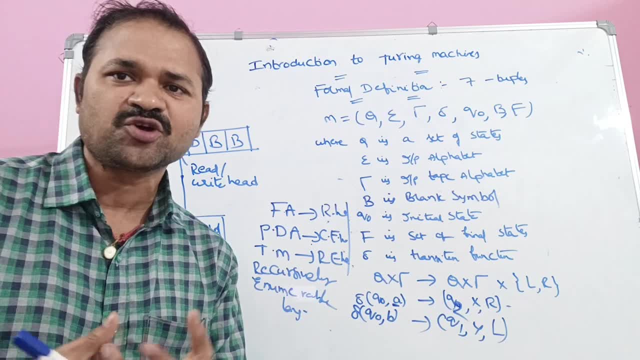 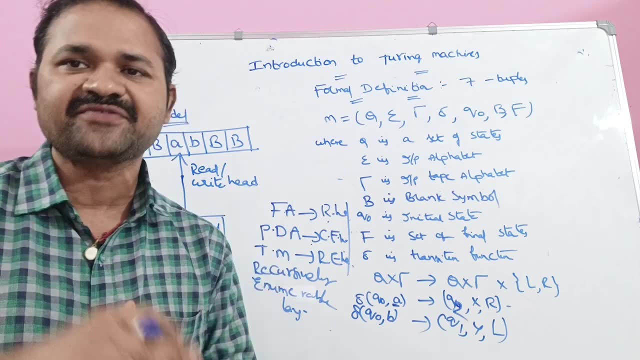 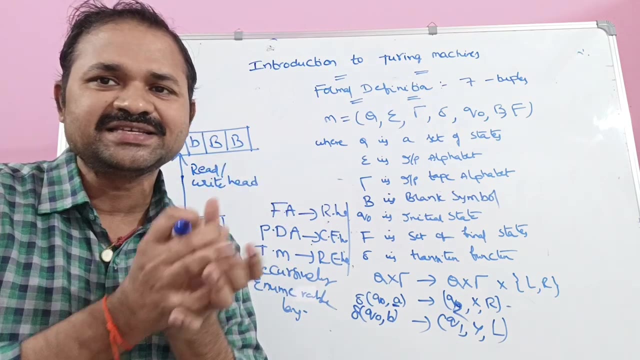 machines. We know that the problem with finite automata is: finite automata has limited amount of memory. So if you want to store some complex languages, then we have to go for pushdown automata. Again, pushdown automata recognizes simple languages. If you want to generate 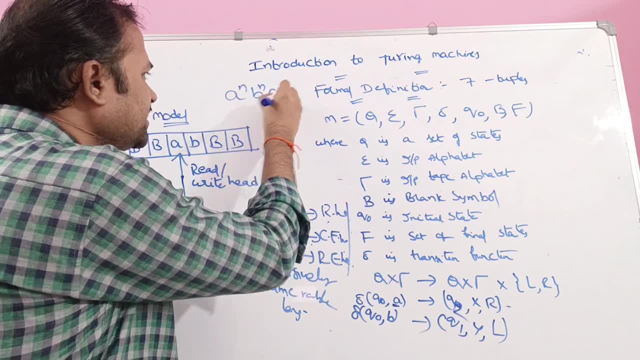 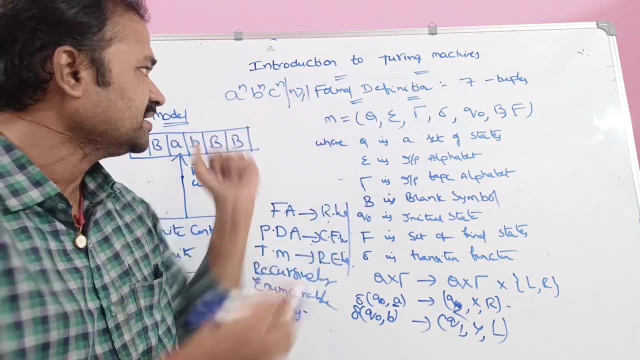 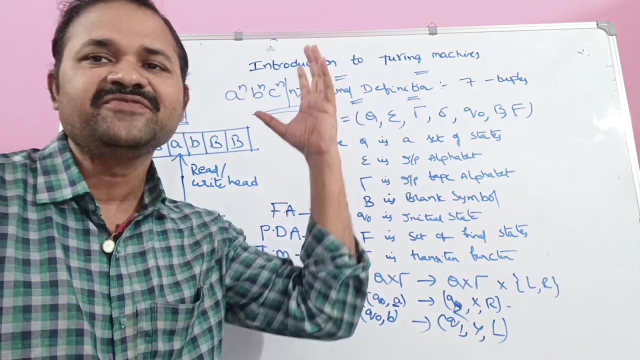 a language like this: a power n, b power n, c, power n such that n greater than or equal to 1. Pushdown automata can't accept this type of language. So if you want to accept a complex language, then we have to go for Turing machine. So Turing machine is a complex. 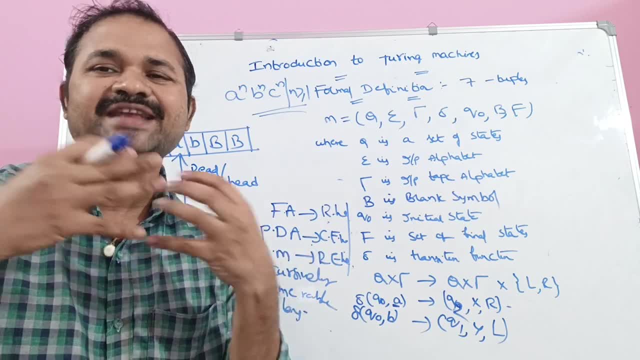 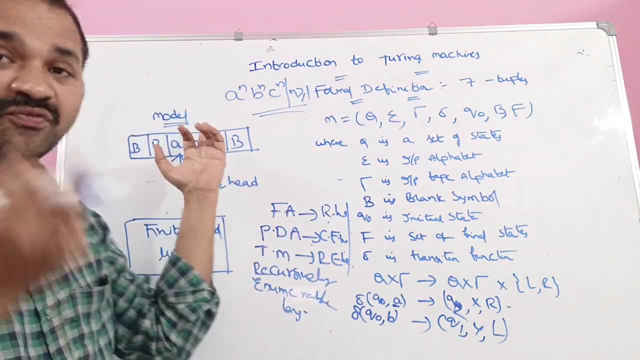 machine. By using Turing machine we can accept any sort of language, any type of language. So in this video we are going to see how to use Turing machine. So in this video we are mainly discussing about the model of the Turing machine, the basic diagram of the Turing. 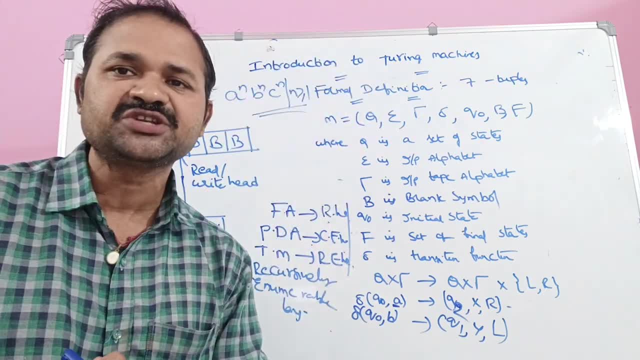 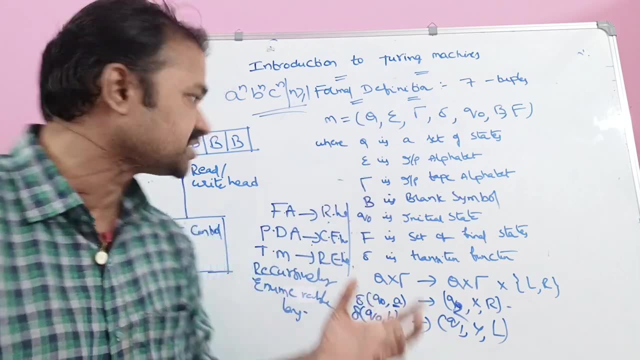 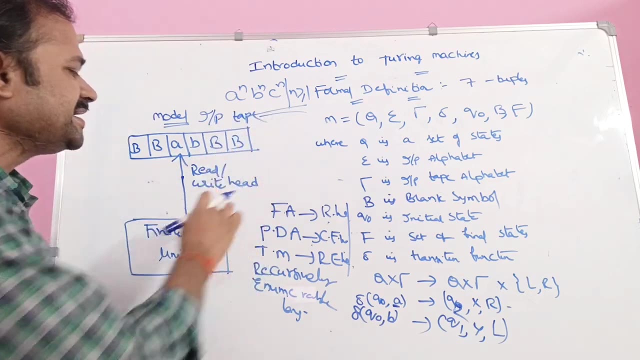 machine as well as the formal definition for the Turing machine. First let us see the model of the Turing machine. So any Turing machine mainly contains three components. The first component is input tape, So this is input tape. The second component is read write head. 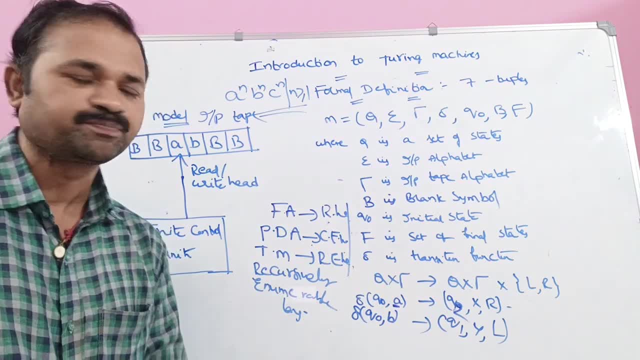 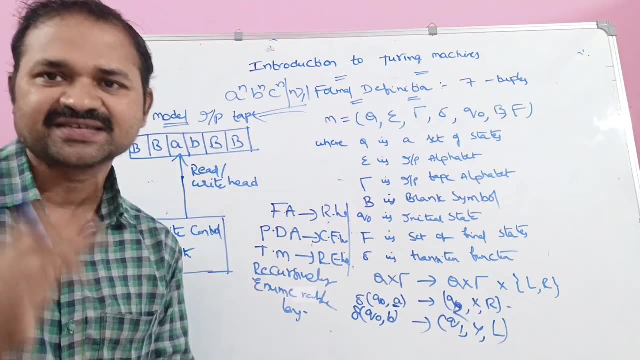 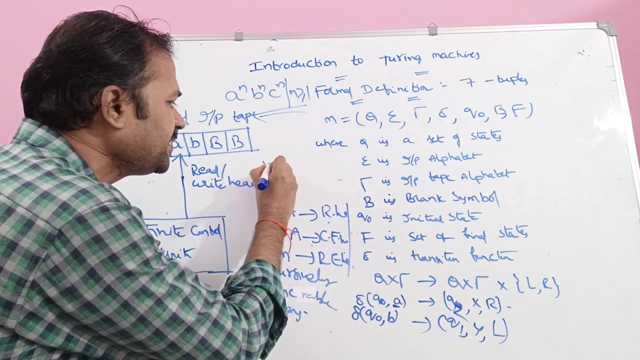 The third one is a finite control unit. First let us see about Turing machine. So this is an infinite input tape. Input tape is divided into number of cells, where each cell can stores one symbol at a time. Here the size of the input tape is infinite, So we can store any. 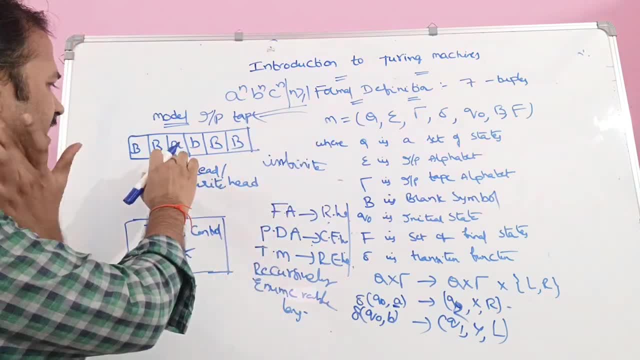 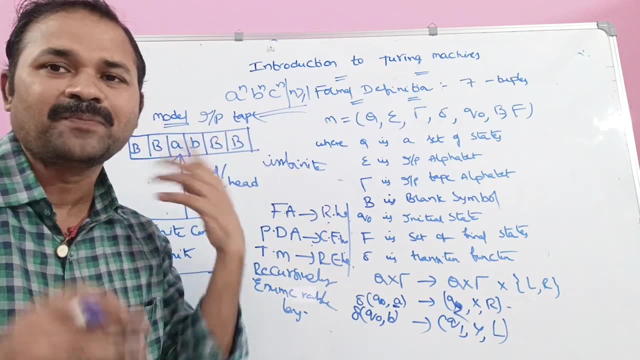 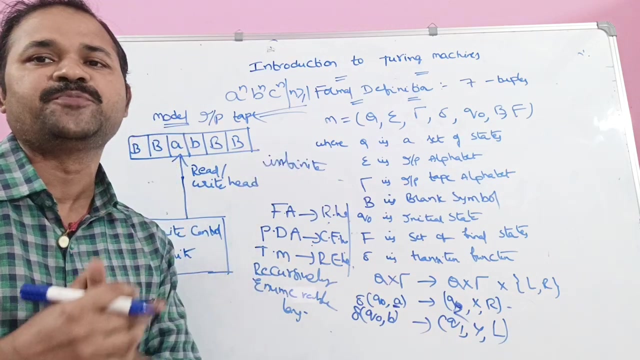 number of symbols in the input tape. Here the input tape contains A and B symbols. So before and after the string we have blank symbols. B stands for blank. So this is the input tape. So we can store any number of symbols in the input. We can store any number of symbols. 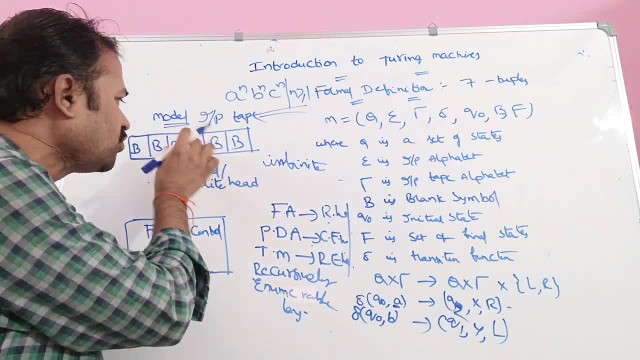 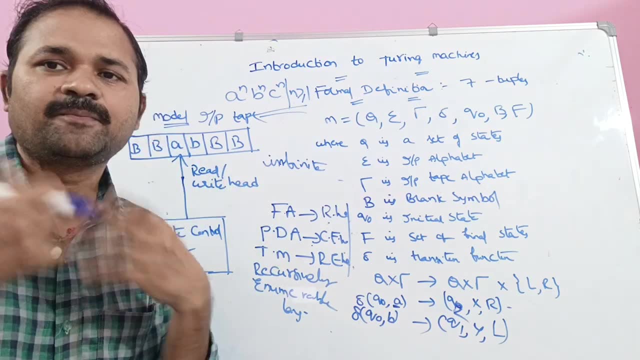 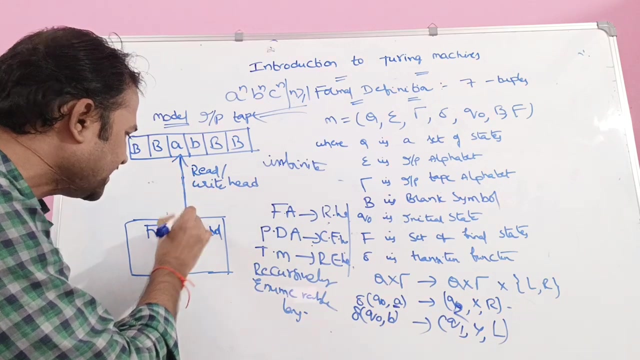 in the input tape. But here the input tape contains only two symbols, A and B, And before and after the A and B we have plenty of blank symbols Here. the next component is read write head. So by using read write head we can perform. 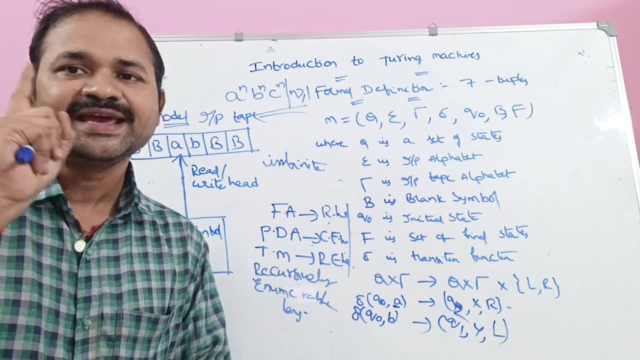 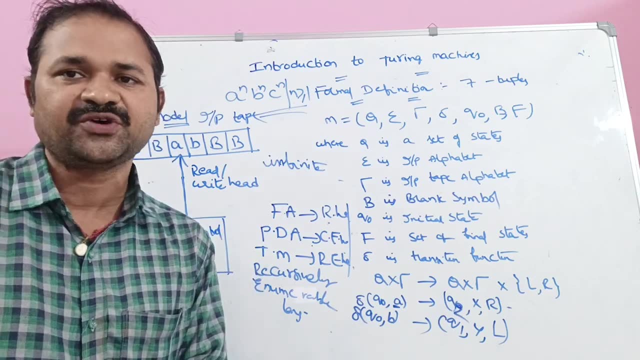 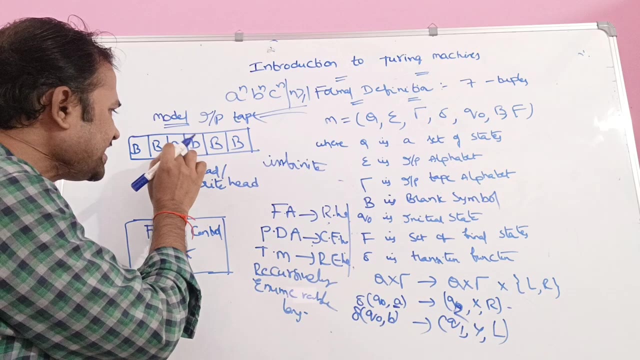 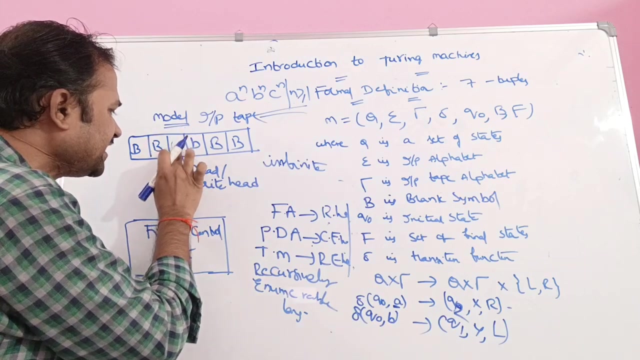 read output. There we can determine the type of Sh loadbar. So here we have read, write led So we can make one type of Sh loadbar and then also write new type ofピ so we can transfer to another type of saber as our c utterly write. So after 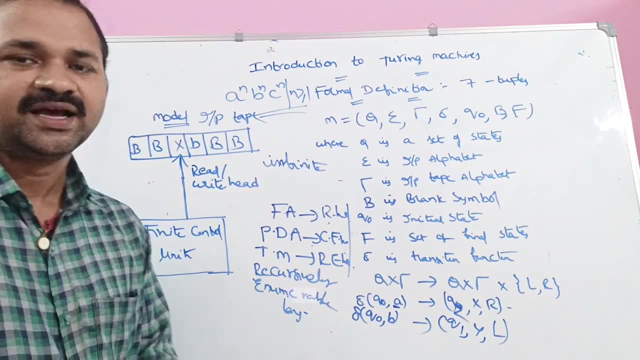 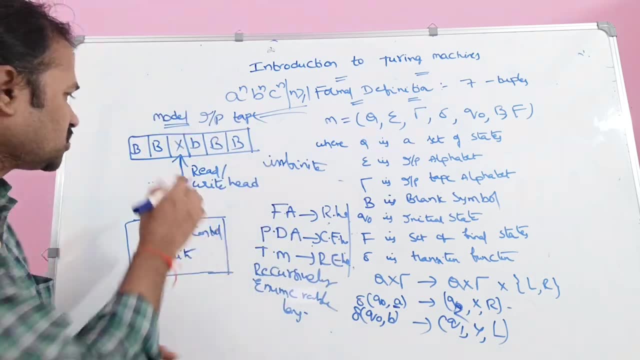 the True type of Sh loadbar is displayed. the R suite led will look out. we can define 3.5 bar series with the help of the read-write head. we can move either from left to right or from right to left. So let the read-write head is at this location, So after that we can move to its right position. 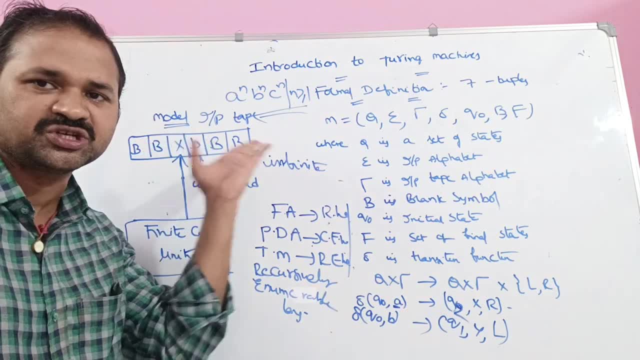 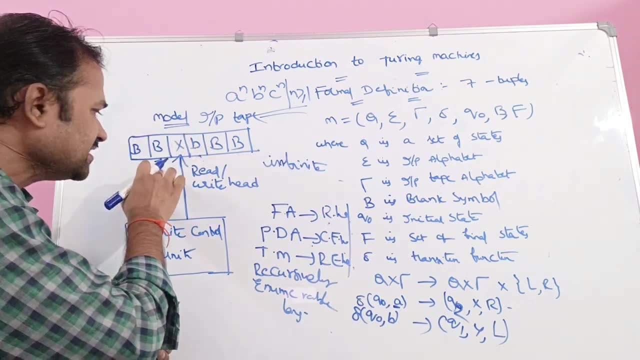 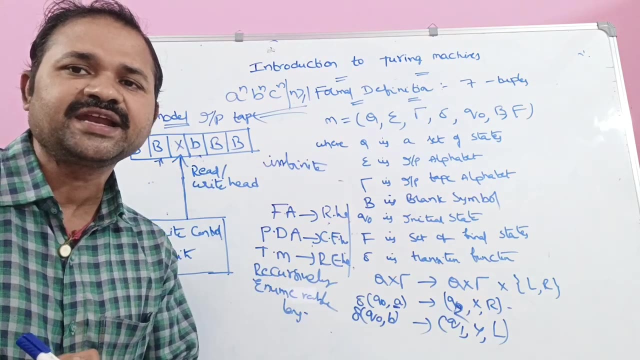 So that means we can move to its next position right, position B- or we can move the read-write head towards its left also. So if we move towards the left, then the read-write head will be at this position. okay, So this is about read-write head. So what is the advantage of the read-write head? 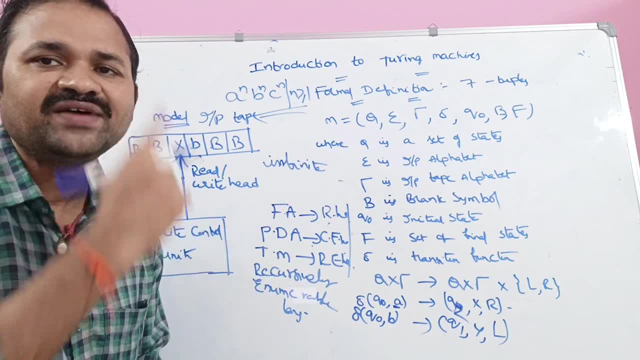 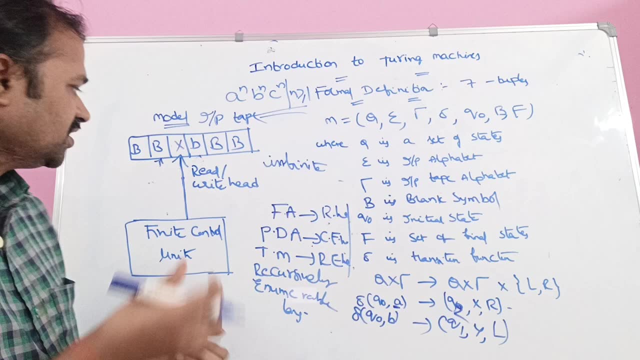 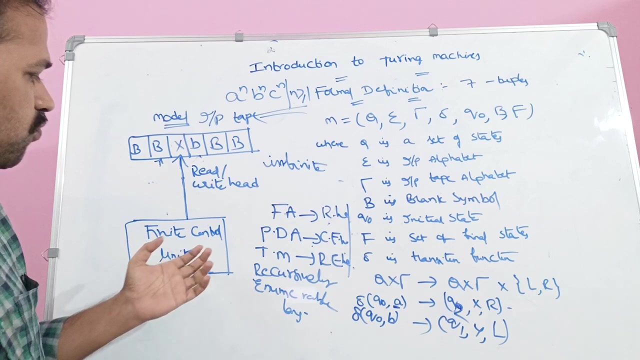 It is useful for reading the data, for reading it only once in a decade, or we can perform the write operation, We can change the content of the cell and after that we can move the read-write head either from left to right or from right to left also okay, So next, here we have finite control. 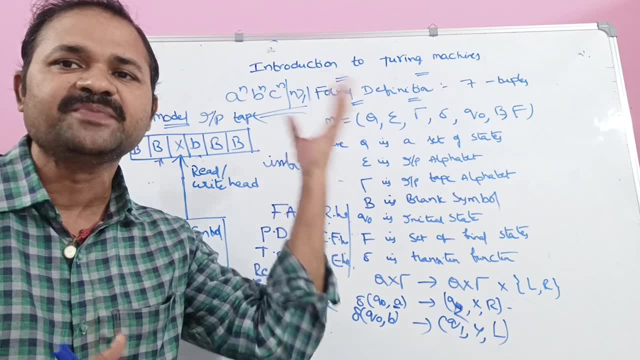 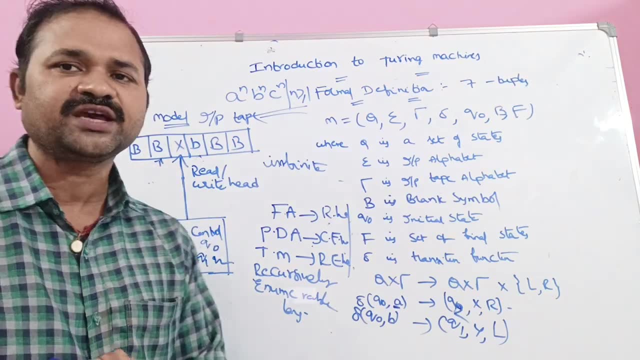 unit. So it contains all the states present in the mission, So that we have five states. So all the five states are present in the finite control unit. okay, Now let us see see the formal definition of the Turing machine. A Turing machine is defined with the help. 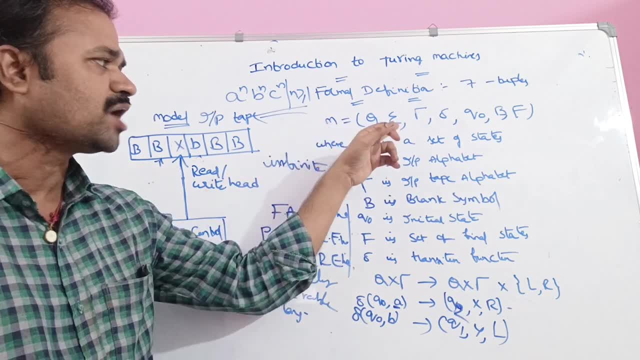 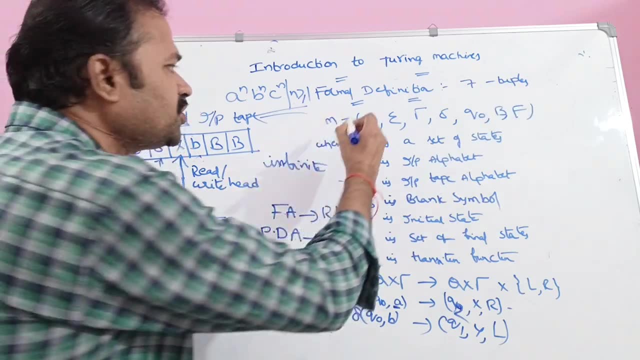 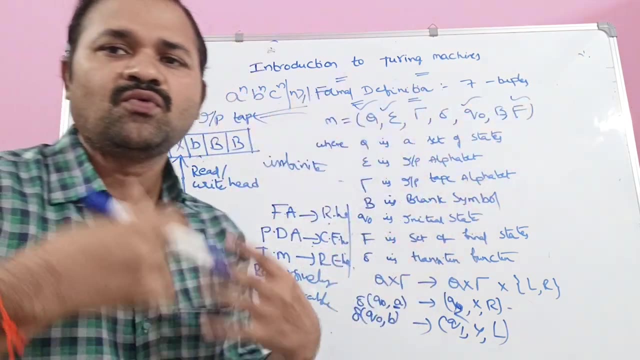 of several tuples. m is equal to q, sigma, tau, delta, q0, b, f. So here we know about q, sigma and q0 and f. So all these four tuples are similar to what we saw in finite. 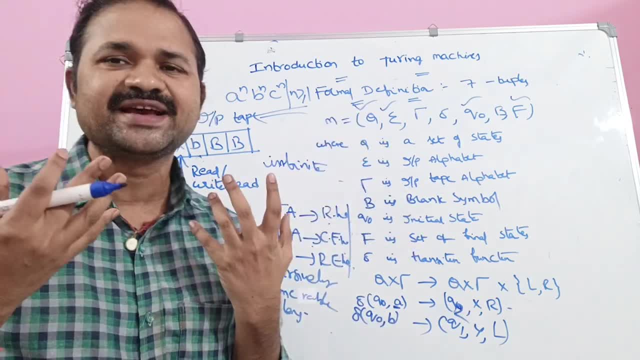 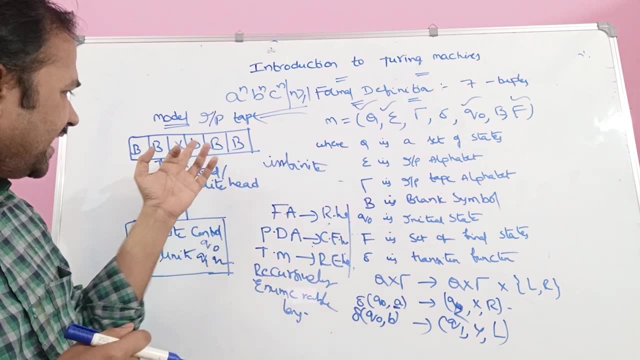 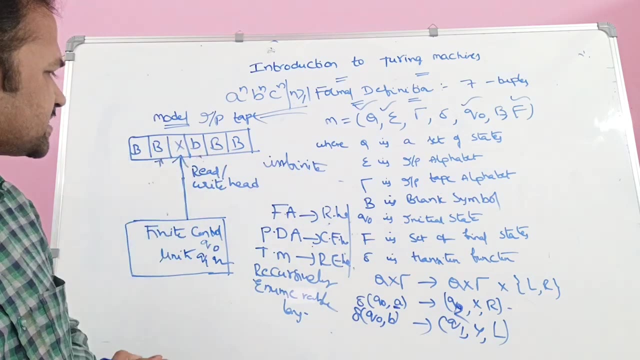 automata and push-door automata. So q means a set of states, sigma means input alphabet. Here the input alphabet contains a and b, as well as x and y and b. also Input alphabet contains a- b symbols. Input alphabet mainly contains for a- b symbols, Input alphabet. 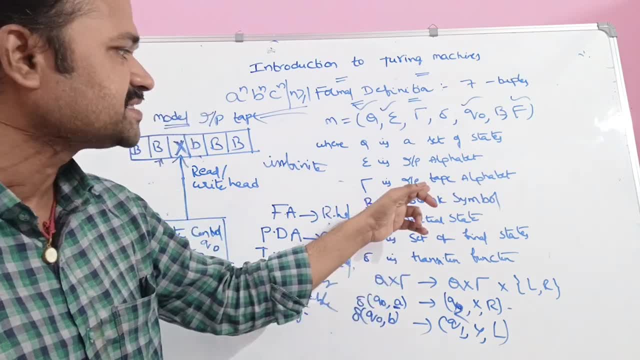 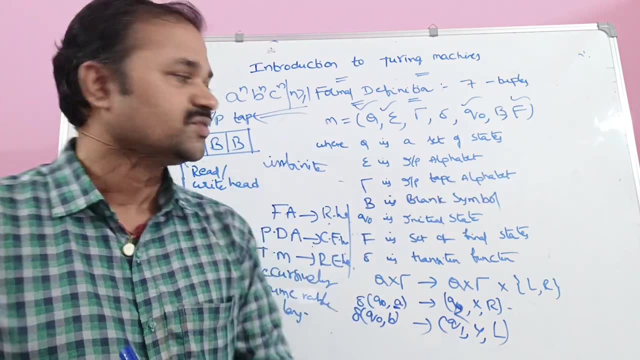 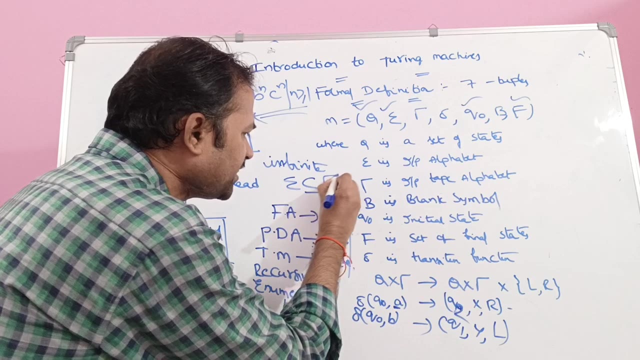 and the next one is tau. Tau is called as the tau. Let us see about tau. So tau is called as tape alphabet, input tape alphabet. So what is input tape alphabet Here? sigma is a subset of input tape alphabet. Sigma means input alphabet. So if you take this, 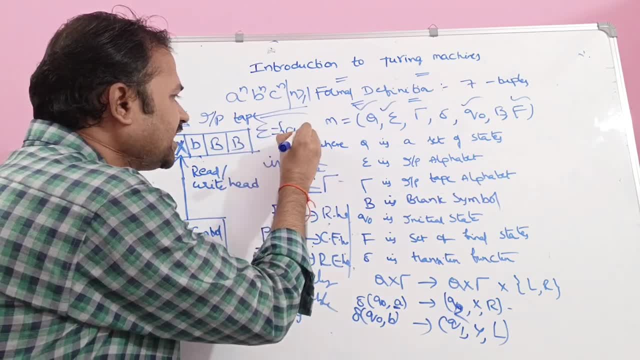 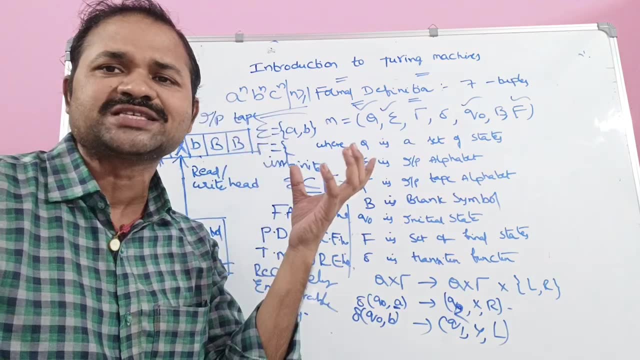 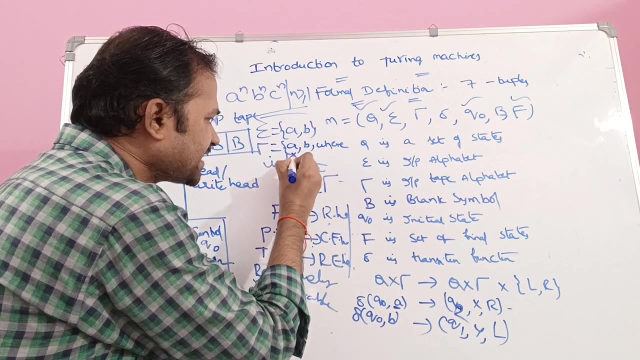 problem. sigma contains only two symbols. They are a and b, Whereas tau. tau means tape alphabet. Tape alphabet means all the symbols which are present in the input tape, So various. the symbols of the tau are a, b, x, y and b. So a b in place of a, I want. 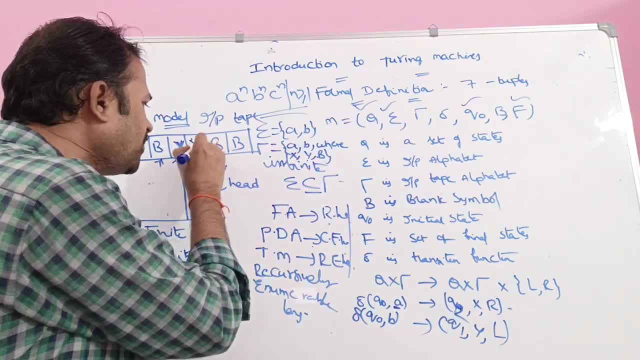 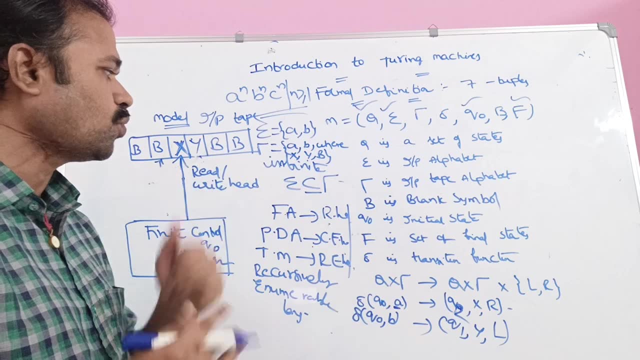 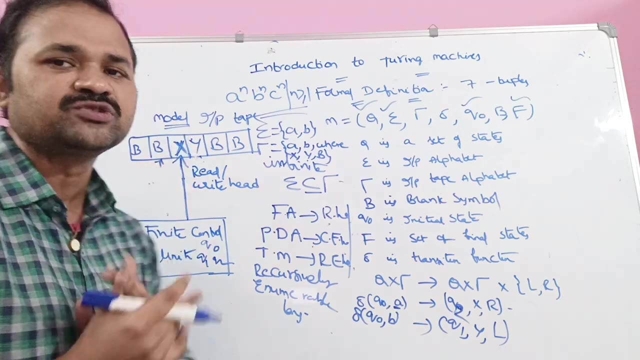 to modify the content as x In place of b. I want to modify the content as y, So tau contains a, b, x, y, as well as black symbols also present in the tau. So tau means tape alphabet, Whereas sigma means input alphabet. Input alphabet contains only two symbols. 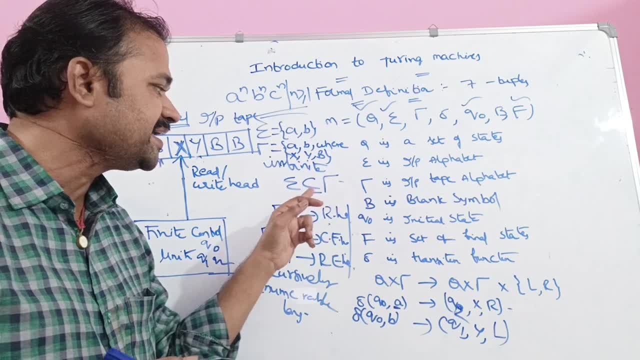 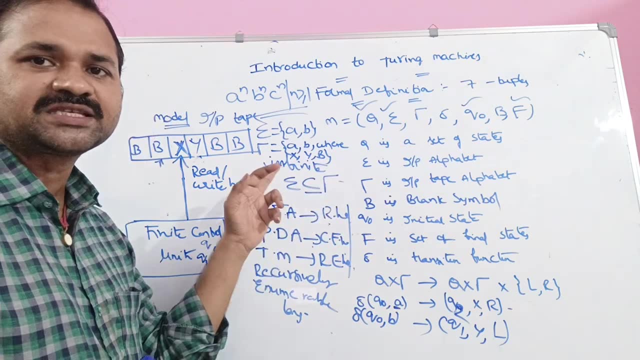 They are a and b. So that is why we can say that Sigma is a subset of tau. That means all the symbols which are present in sigma are present in the tau. Here the sigma contains two symbols. They are a- b. So a- b are present. 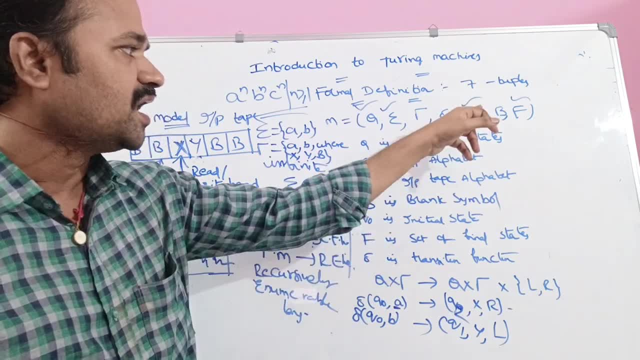 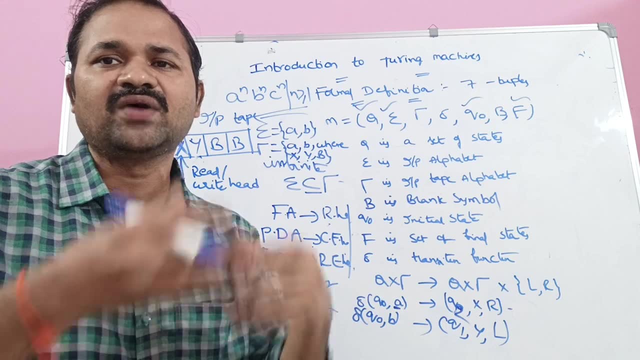 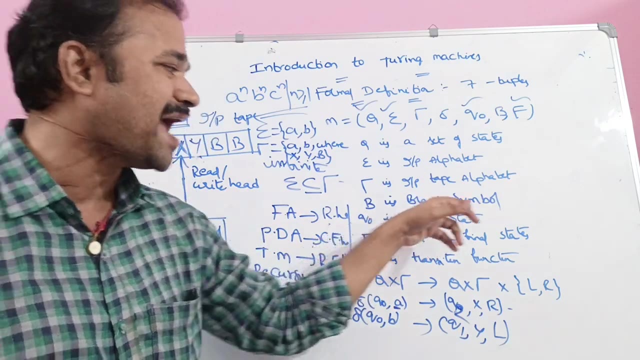 in tau also. Next, here we have q0.. So q0 means initial state, F means a set of final states. So here also we may have a number of final states. So next one is b. b stands for blank symbol. b stands for what? Blank symbol. Blank symbol means a set of initial. 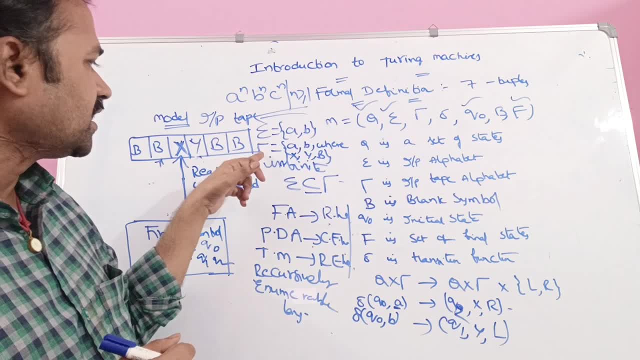 states. So here also we may have a number of final states. So next one is b. b stands for blank symbol, So here also we may have a letter. So here also black symbol is a part of the tape alphabet, So blank symbol is present. in tau also, Blank symbol is present. 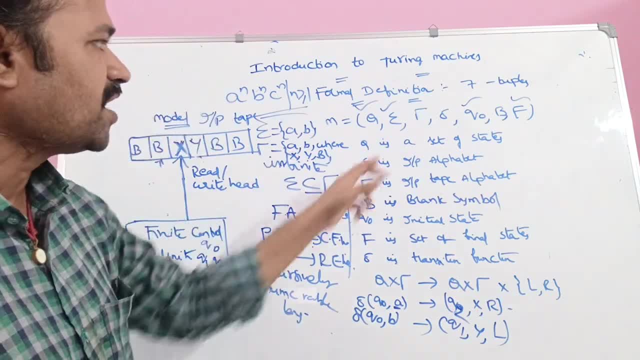 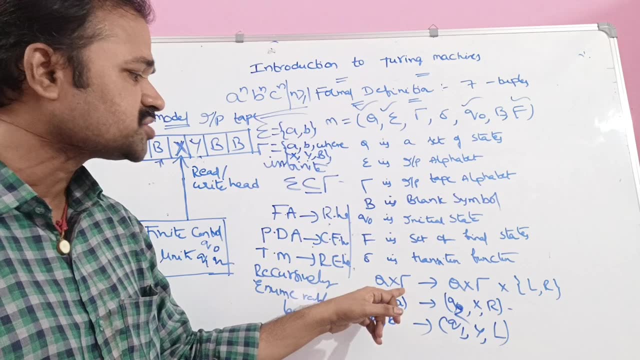 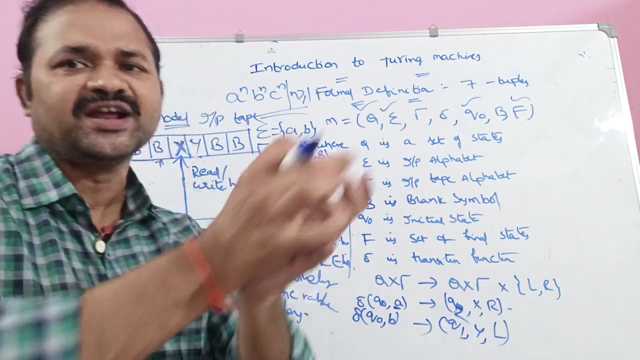 in tau also. So in put on the it also. Next we have one more topple, that is delta. Delta is a transition function which maps from q cross tau to q cross tau. cross l comma r. L means we are moving in left-two directions. 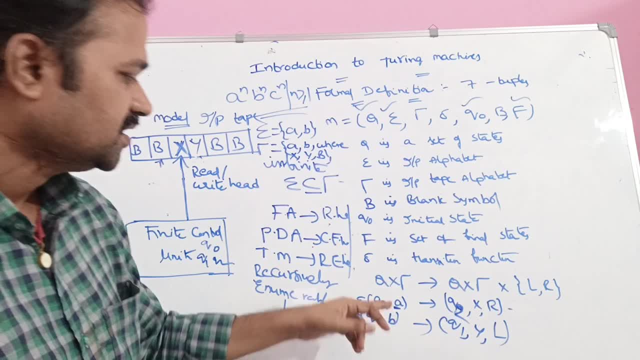 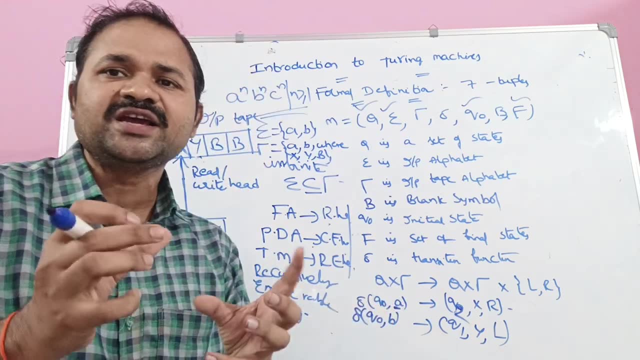 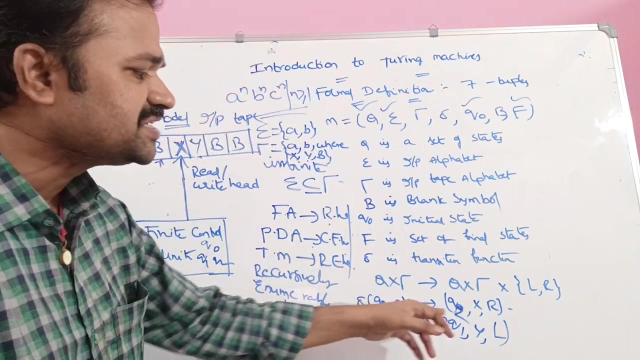 R means we are moving in right-direction. Ok, Jose, let us take it from here. This is So. let us take an example for this delta of let. Q means Q naught, So currently we are at Q naught state. tau means A, So that means if we apply A on Q naught, let us assume that we are moving to. 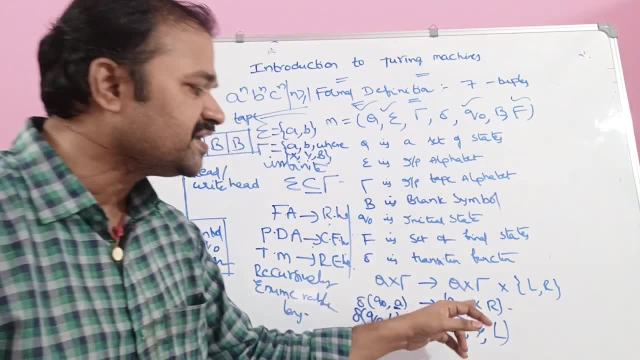 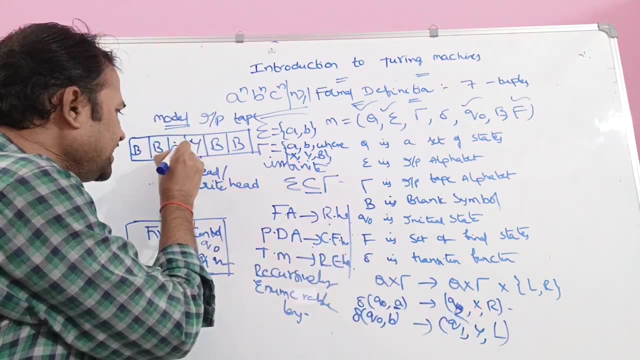 Q2.. So that Q2 is nothing but Q. next one is X. If we read A, then modify the content to X. So here we have A. if we read A on Q, naught, let us modify the content to X. and after reading that, 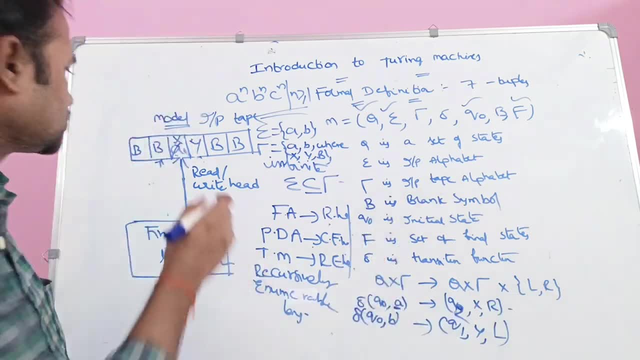 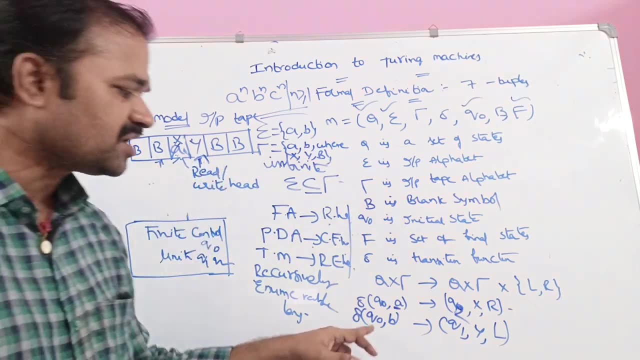 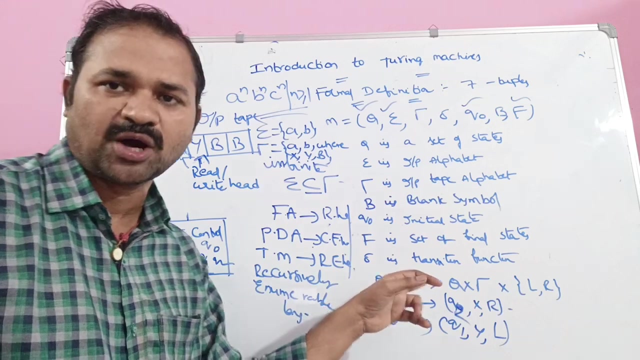 content. let us move the head towards the right. So now the read write head is at this position. So now the read write head is at this position. So let us take one more example: delta of Q naught, comma B. So Q naught means the state, whereas B means tau. So if we apply B on Q naught, 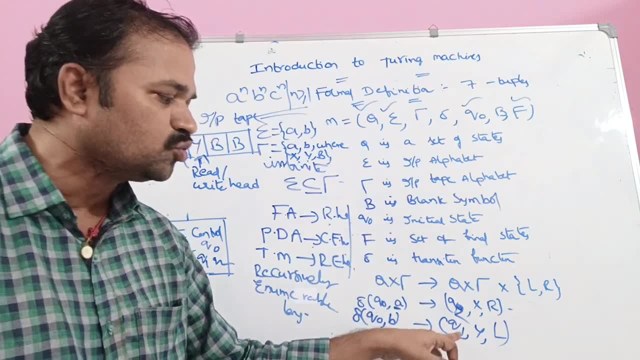 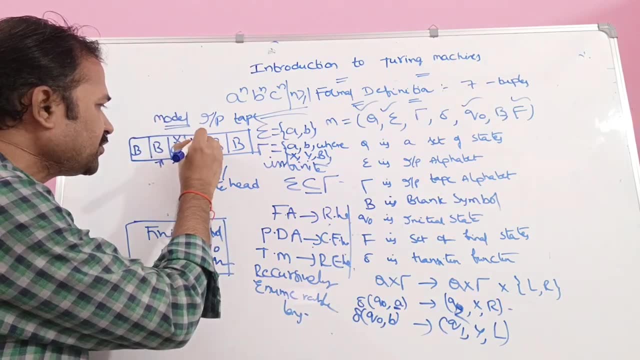 let us assume that B transition, Let us assume that we move to Q1 and modify the content to Y. So if you read B, then modify the content to Y, Then modify the content to Y After reading that, after it is: 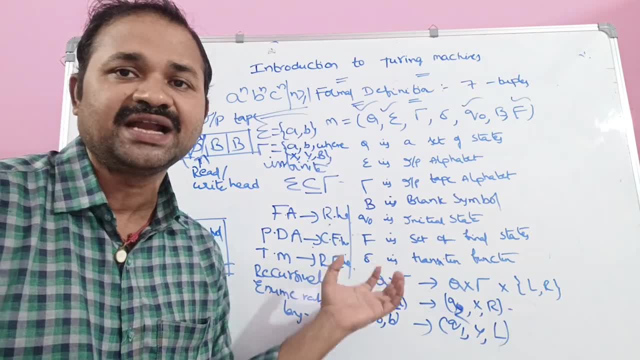 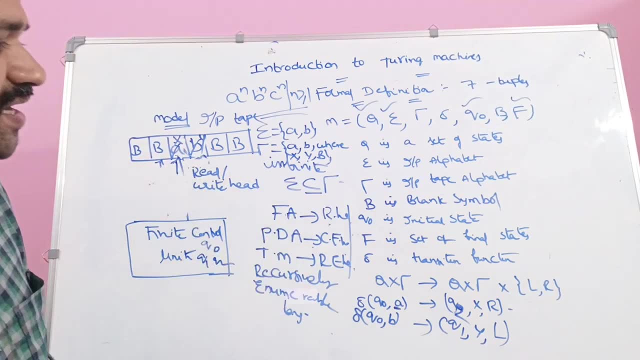 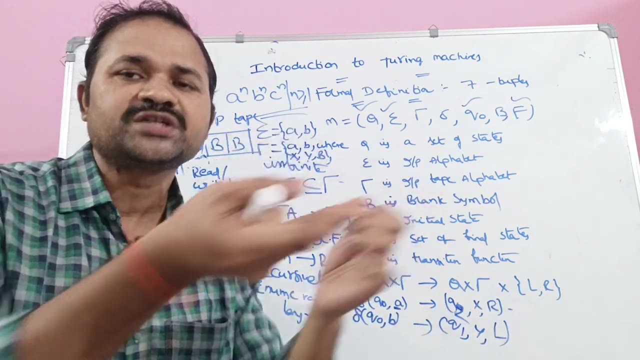 over, then move the read-read head towards the left. So move the read-read head towards the left. So now we have to move towards the left. So likewise we have to specify R or L. So R means we have to move the read-read head towards the right, L means we have to move the. 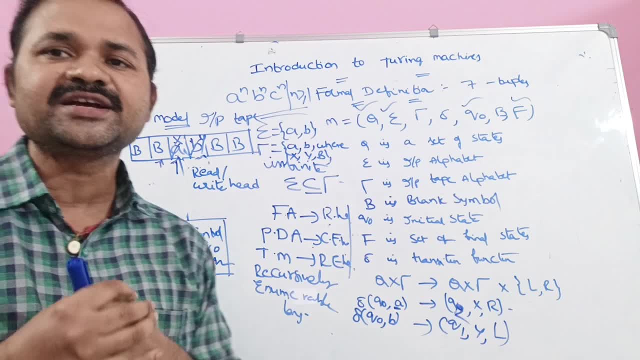 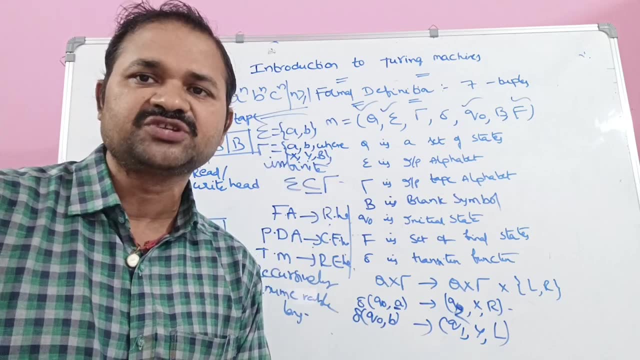 read-read: head towards the left. So this is about introduction to Turing missions, such as model of the Turing machine, diagram of the Turing machine, as well as formal definition of the Turing machine.